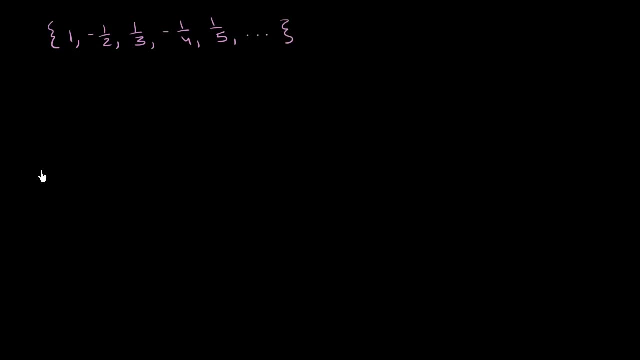 and it just keeps going on and on and on like this, And we could graph it. Let me draw our vertical axis, So I'll draft this as our y-axis and I'm going to graph: y is equal to a sub n And let's make this our horizontal axis. 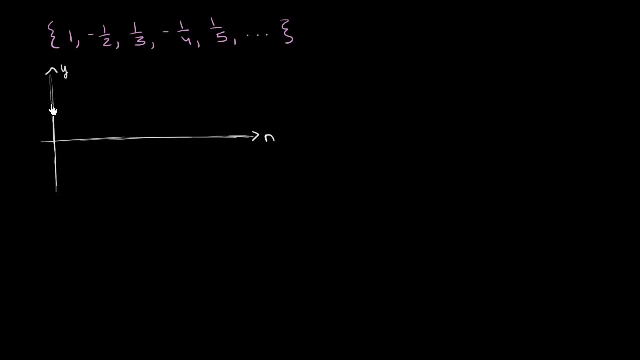 where I'm going to plot our n's. So this right over here is our n's. and let's say this right over here is positive 1.. This right over here is negative 1. This would be negative 1 half. This would be positive 1 half. 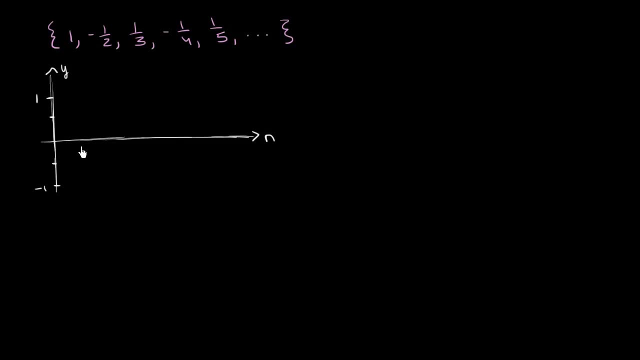 And I'm not drawing the vertical and horizontal axes at the same scale, just so that we can kind of visualize this properly. But let's say this is 1,, 2,, 3,, 4,, 5,, 6,, 7,, 8,, 9,, 10.. 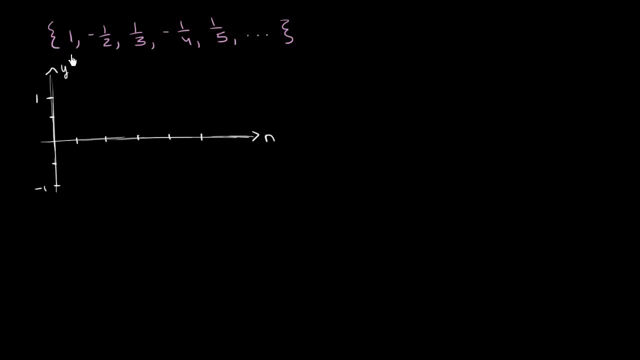 And I could keep going on and on and on. So we see here that when n is equal to 1, a sub n is equal to 1.. So this is right over there. So when n is equal to 1, a sub n is equal to 1.. 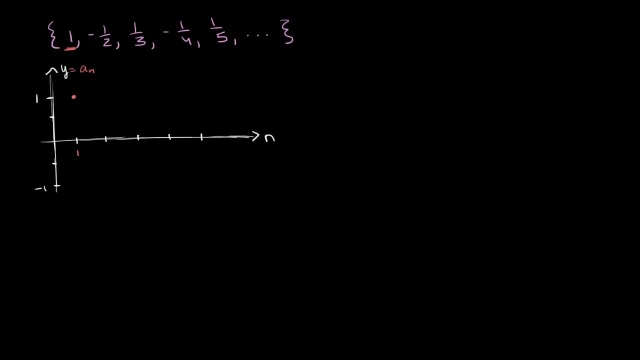 So this is: y is equal to a sub n. Now, when n is equal to 2, we have: a sub n is equal to negative 1 half. When n is equal to 2, a sub n is equal to negative 1 half. 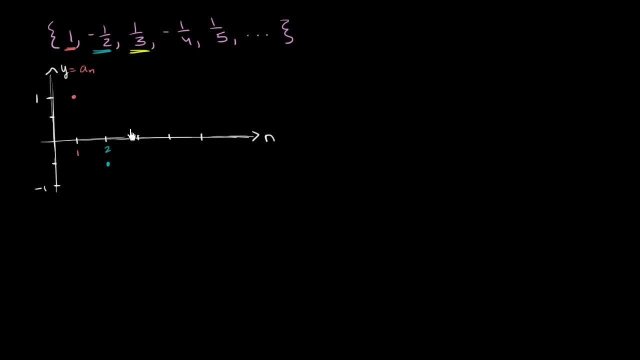 When n is equal to 3, we have a sub n is equal to negative 1. third, When n is equal to 4, a sub n is equal to negative 1. fourth, which is right about there. And then when n is equal to 5, a sub n is equal to positive 1. 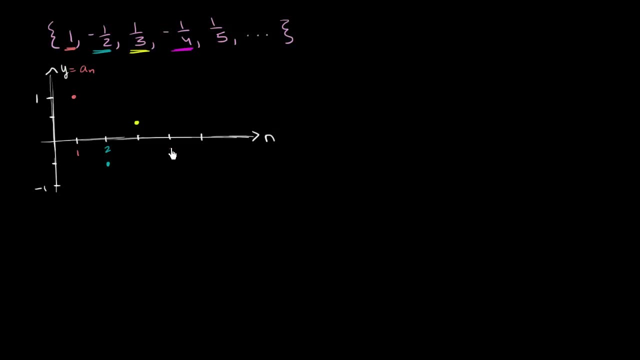 fifth, which is maybe right over there, And we keep going on and on and on. So you see the points. they kind of jump around But they seem to be getting closer and closer to each other. So we see that when n is equal to 5, a sub n is equal to positive. 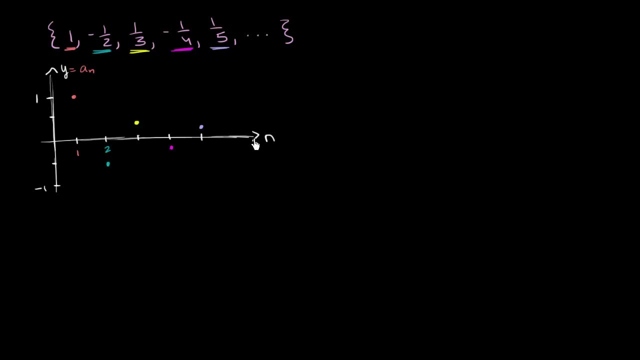 1. fifth, which is maybe right over there, Closer and closer and closer to 0,, which would make us ask a very natural question: What happens to a sub n as n approaches infinity, Or another way of saying that is: what is the limit? 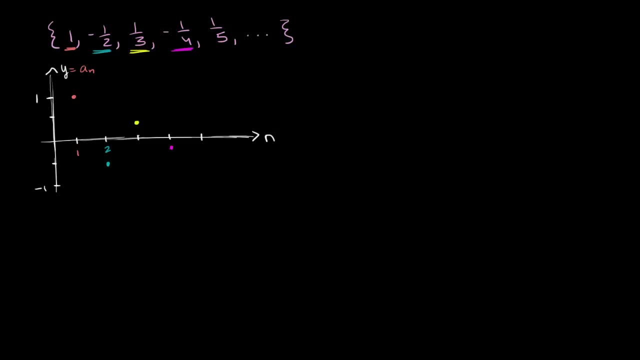 which is right about there. And then when n is equal to 5, a sub n is equal to positive 1. fifth, which is maybe right over there. And we keep going on and on and on. So you see the points. they kind of jump around. 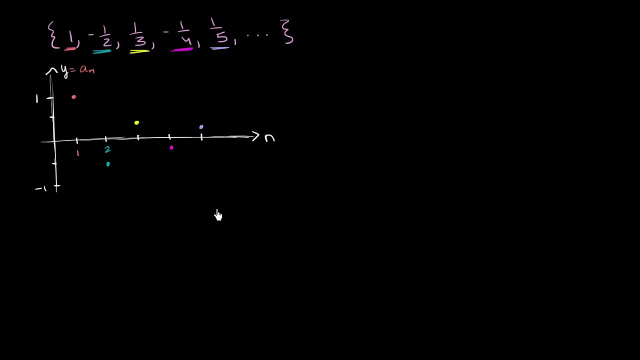 but they seem to be getting closer and closer and closer to 0,, which would make us ask a very natural question: What happens to a sub n as n approaches infinity? Or another way of saying that is: what is the limit of a sub n as n approaches infinity? 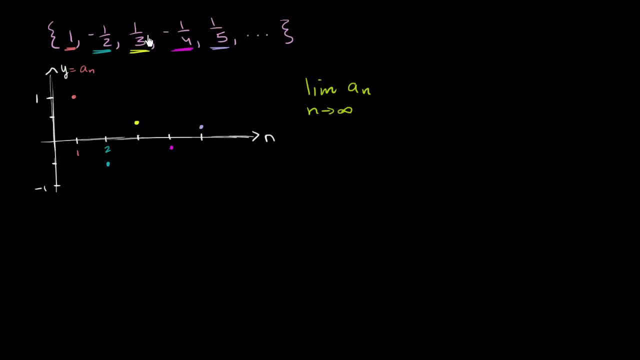 Well, let's think about if we can define a sub n explicitly. if we can, If we can define the sequence explicitly. So we can define the sequence as a sub n, where n starts at 1 and goes to infinity, with a sub n equaling. 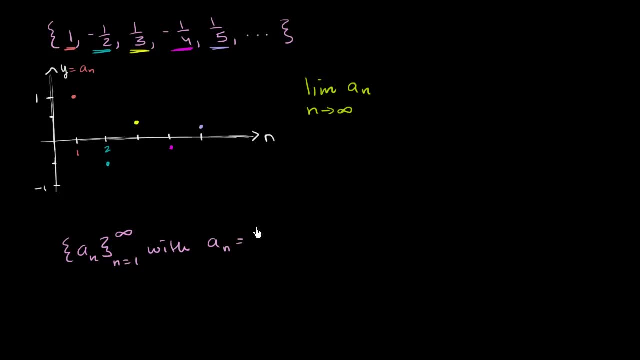 What does it equal? Well, if we ignore a sign, for a second it looks like it's just 1 over n. But then we seem like we oscillate in signs. We start with a positive, then a negative. positive, negative. 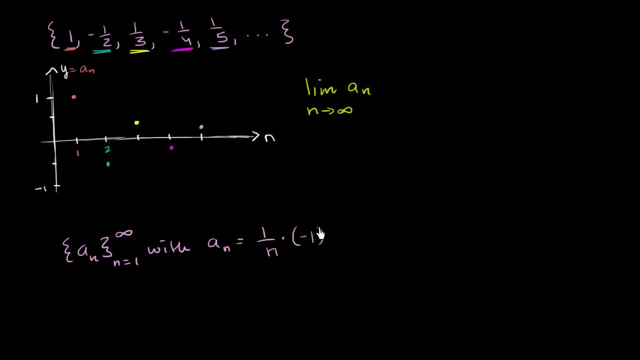 So we could multiply this: times negative 1 to the. let's see: if we multiply it times negative 1, negative 1 to the n, then this one would be negative and this one would be positive. But we don't want it that way. 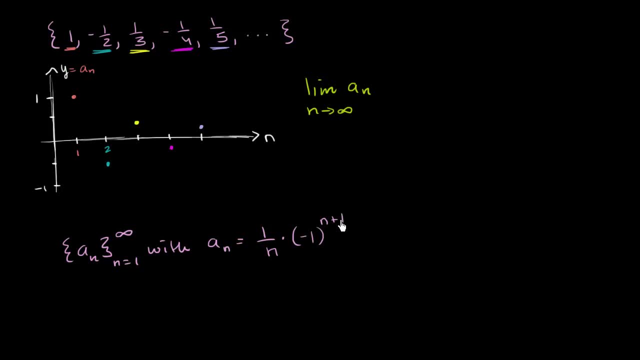 We want the first term to be positive, So we could say negative 1 to the n plus 1 power And you can verify this works. When n is equal to 1, you have 1 times negative 1 squared, which is just 1.. 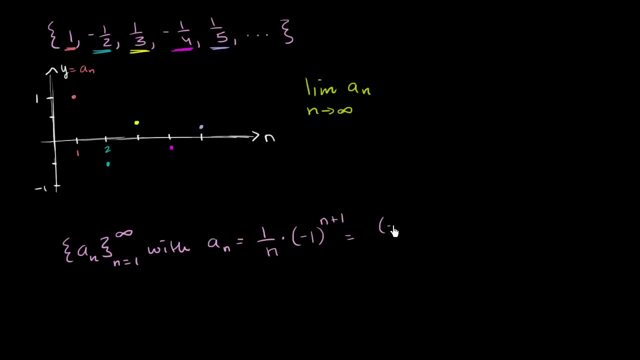 And they'll work for all the rest. So we could write this as equaling negative 1 to the n plus 1 power over n, And so asking what the limit of a sub n as n approaches infinity is is equivalent to asking: 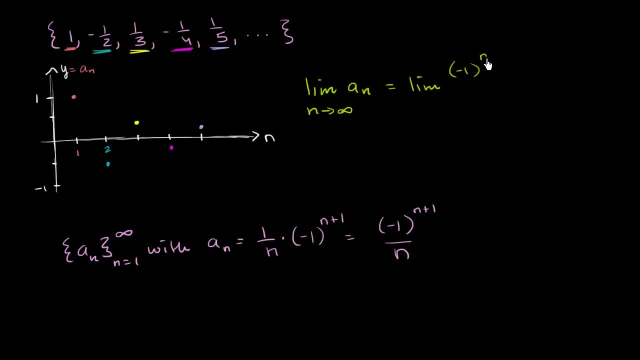 What is the limit of negative 1 to the n plus 1? power over n as n approaches infinity is going to be equal to Remember a sub n. this is just a function of n. It's a function where we're limited right over here. 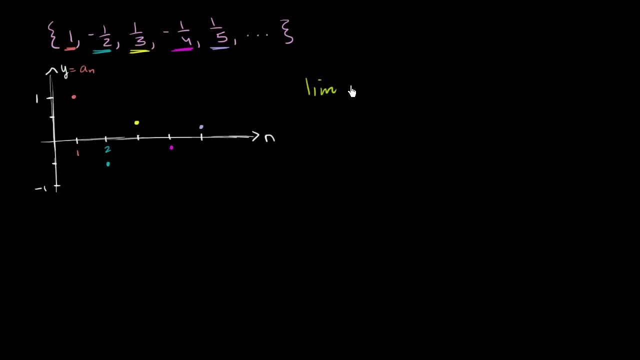 Let me do this in a new color. What is the limit of a sub n as n approaches infinity? Well, let's think about if we can define a sub n explicitly, if we can define the sequence. So we can define the sequence as a sub n where n starts at 1. 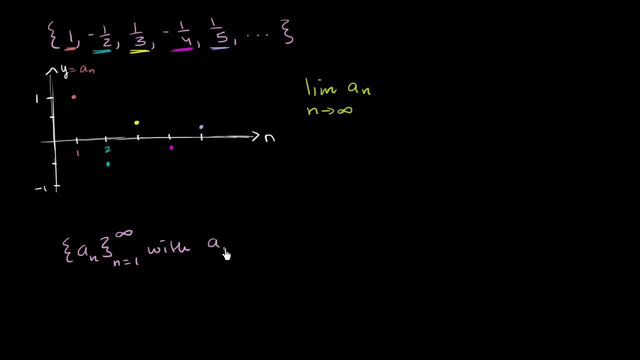 and goes to infinity with a sub n equaling. What does it equal? Well, if we ignore a sign for a second, it looks like it's just 1 over n. But then we seem like we oscillate in signs: We start with a positive, then a negative. positive, negative. 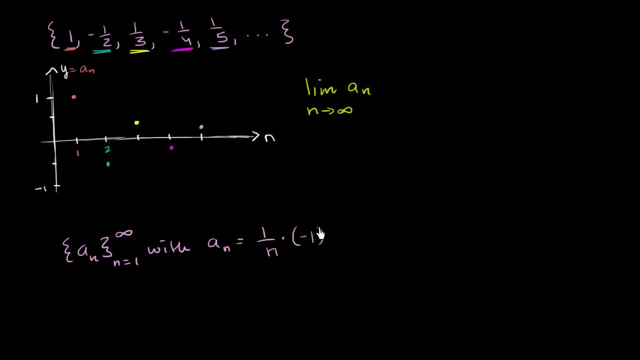 So we could multiply this times negative 1 to the n. Let's see: if we multiply it times negative 1 to the n, then this one would be negative and this one would be positive. But we don't want it that way. 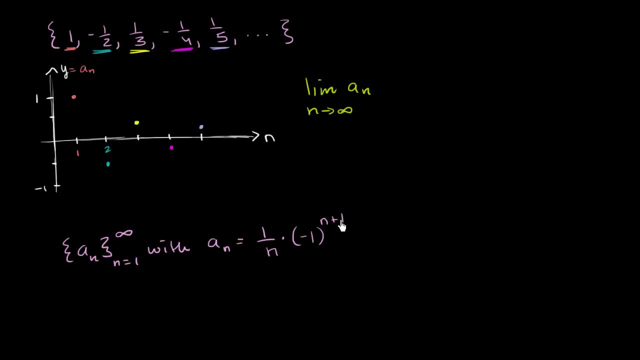 We want the first term to be positive, So we could say negative 1 to the n plus 1 power And you can verify this works. When n is equal to 1, you have 1 times negative 1 squared, which is just 1.. 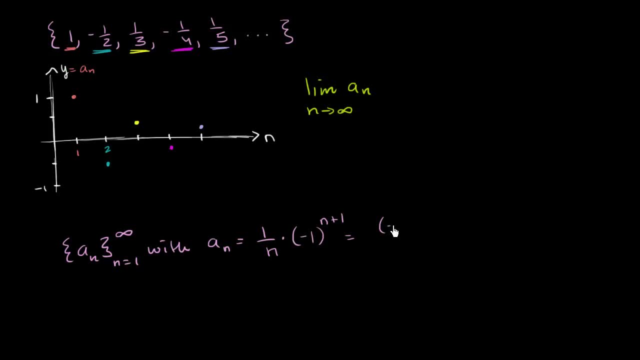 And they'll work for all the rest. So we could write this as equaling negative 1 to the n plus 1 power over n, And so asking what the limit of a sub n as n approaches infinity is is equivalent to asking what is the limit. 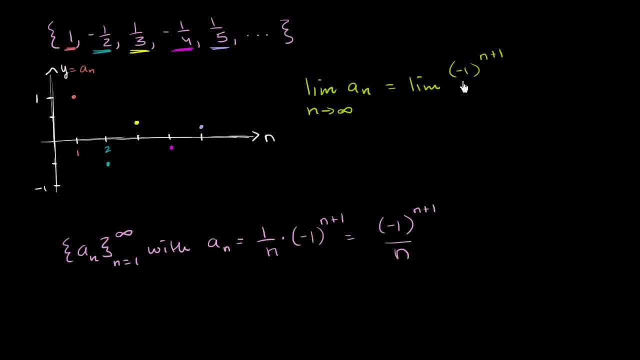 The limit of negative 1 to the n plus 1 power over n. as n approaches infinity is going to be equal to Remember a sub n. this is just a function of n. It's a function where we're limited right over here. 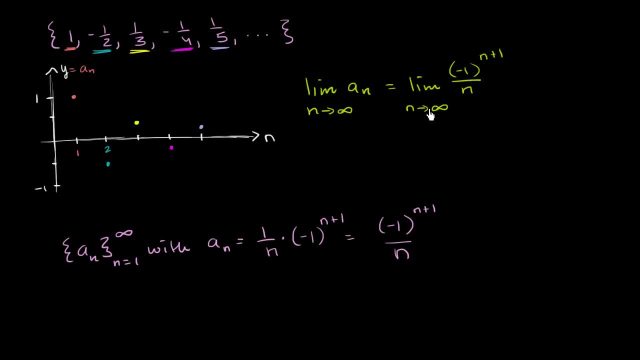 to positive integers as our domain. But this is still just a limit, as something approaches infinity- And I haven't rigorously defined it yet, but you can conceptualize what's going on here. As n approaches infinity, the numerator is going to oscillate between positive and negative 1.. 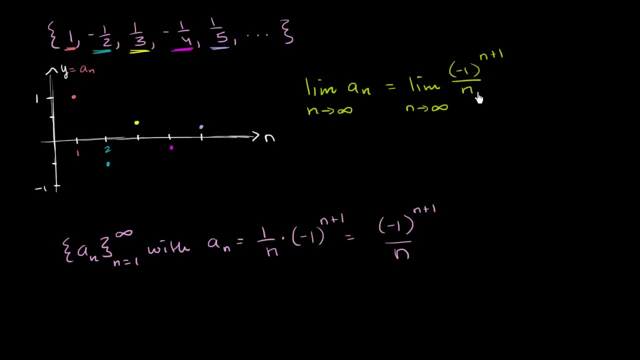 But this denominator is going to oscillate between positive and negative 1. The denominator is just going to get bigger and bigger and bigger and bigger. So we're going to get really, really, really, really small numbers, And so this thing right over here is going to approach 0..